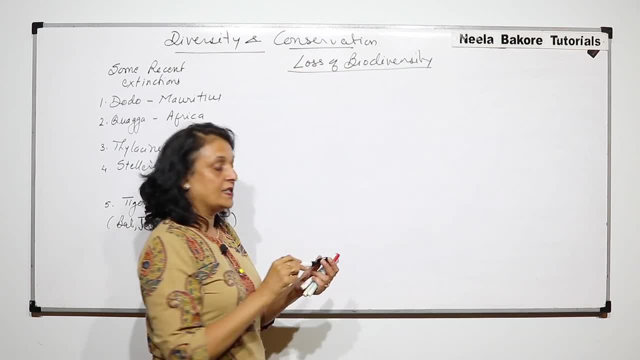 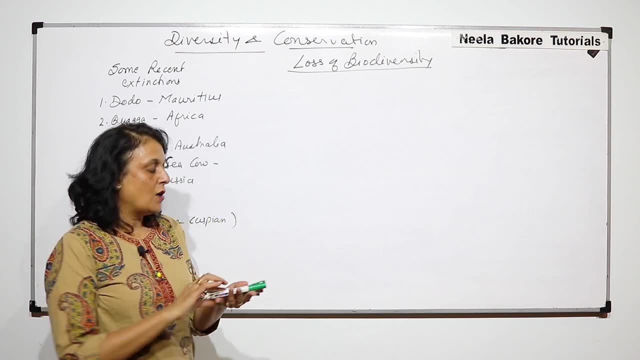 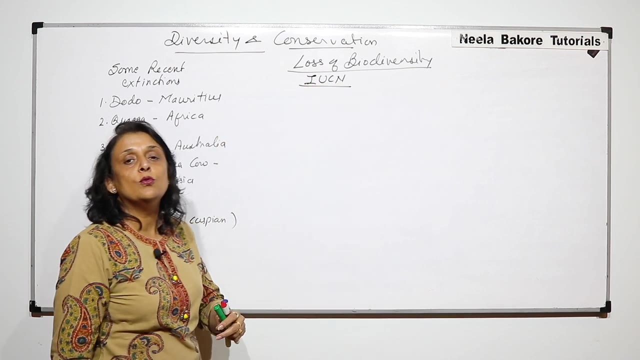 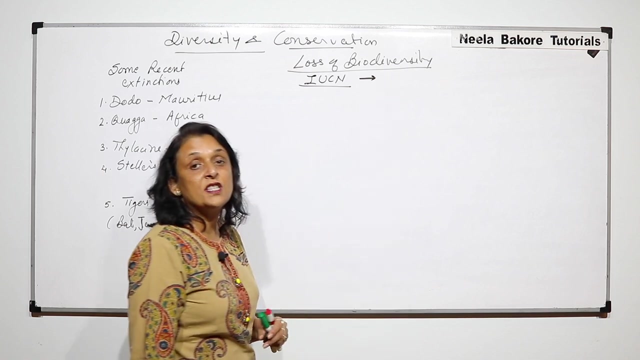 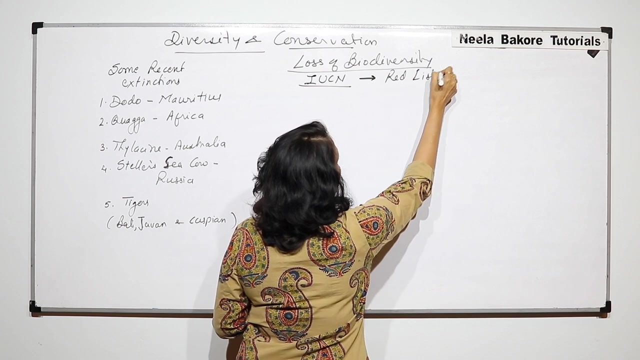 But before we talk about the causes which are responsible for loss of biodiversity, we need to understand few things. According to International Union for Conservation of Nature, there is a list which is published, and this list is known as the Red List, or sometimes it is also known as the Red Book. 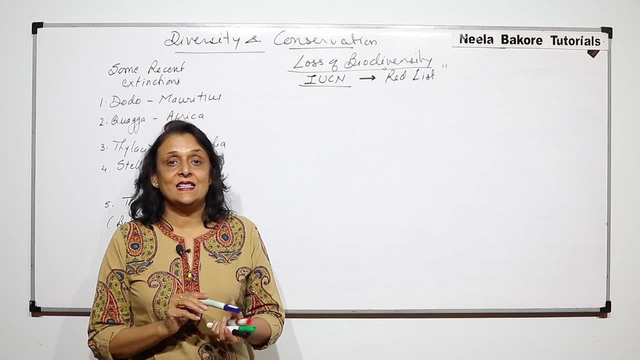 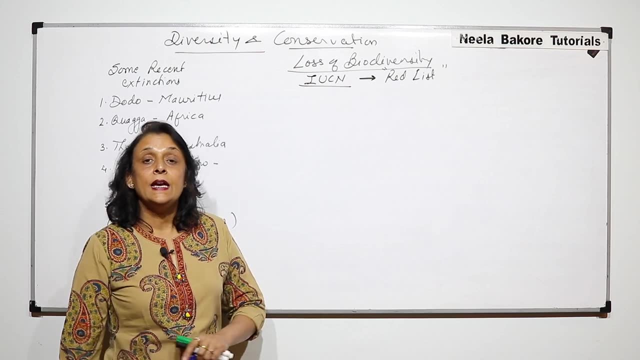 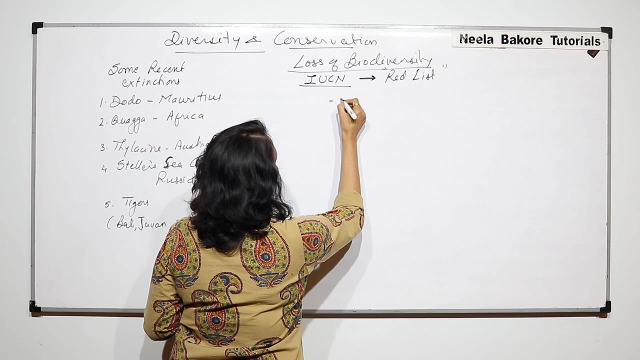 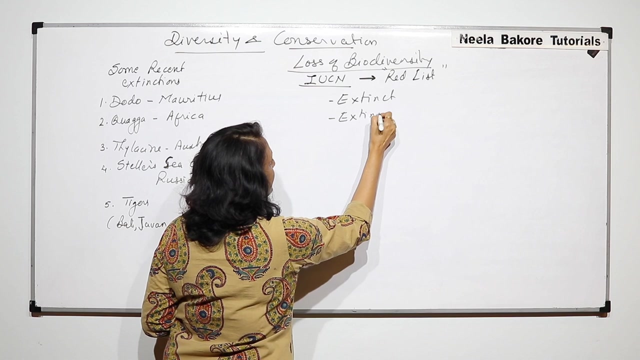 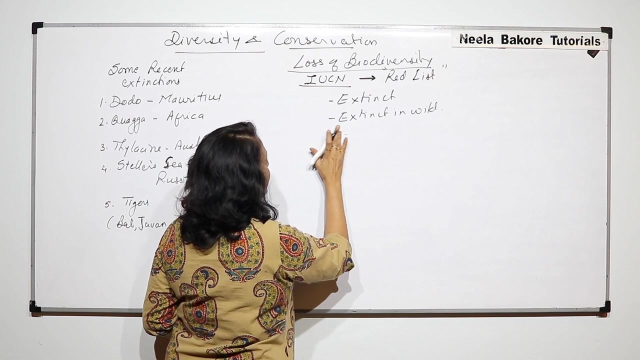 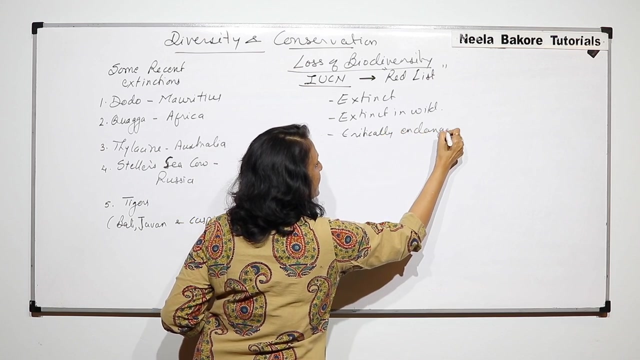 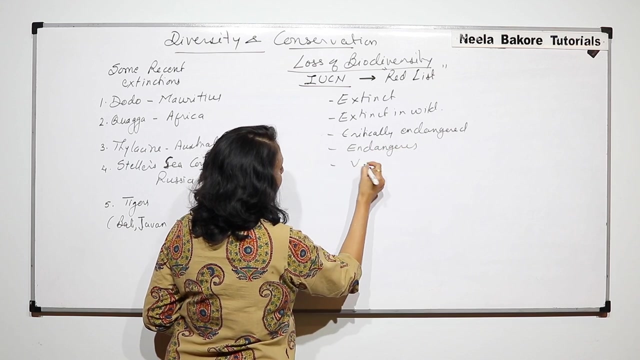 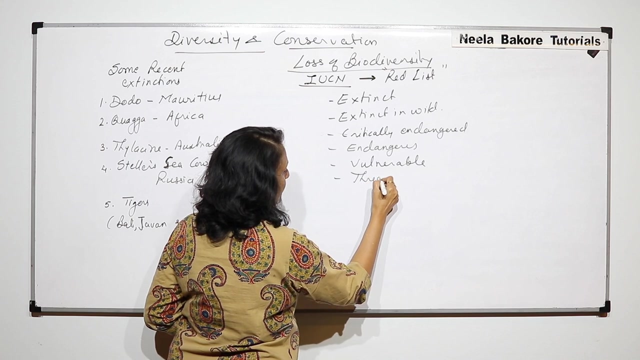 The list contains some organisms belonging to kingdom, animalia, plantae and fungi in various categories, And the categories which are mentioned are extinct, then extinct in wild, critically endangered, then endangered, vulnerable and threatened. Now, what exactly is meant by these categories is 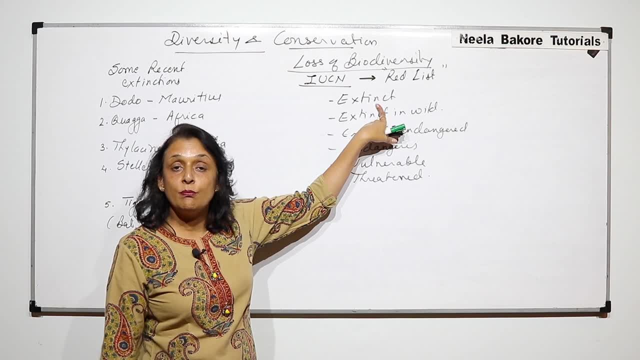 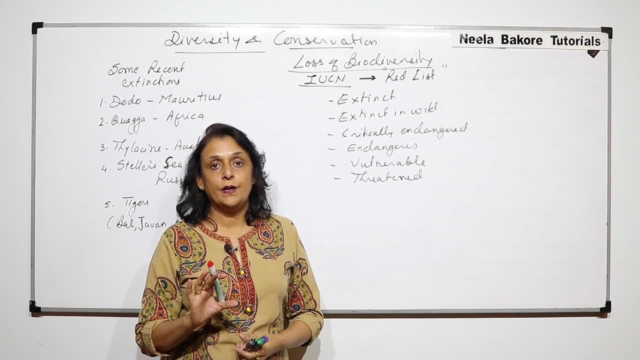 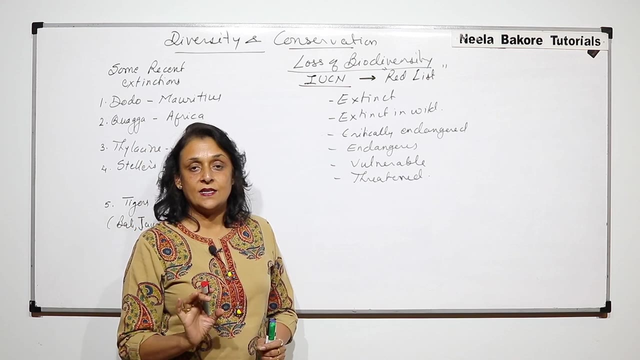 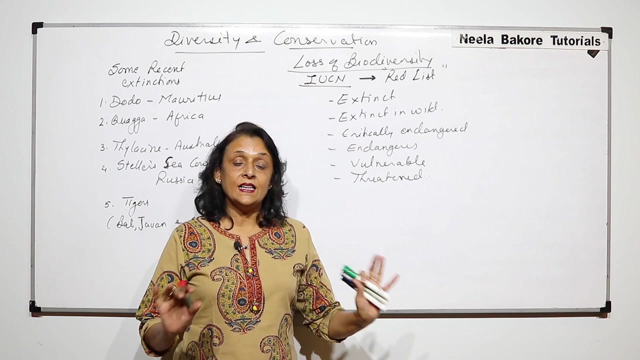 when we say extinct, that means no organism of that particular species exists in the world. It can be a plant, it can be an animal, it can be a fungus, But no animal exists. So then we put it in this category: Extinct in wild, that means they are extinct in the natural habitat. 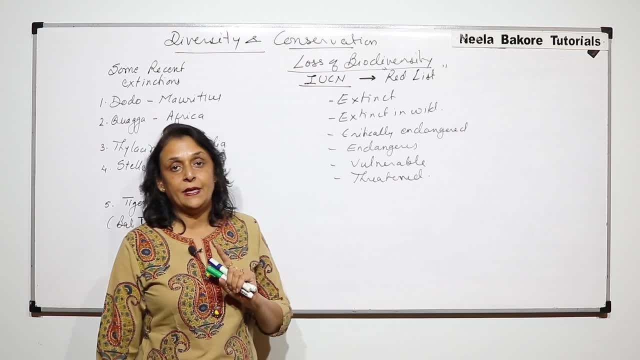 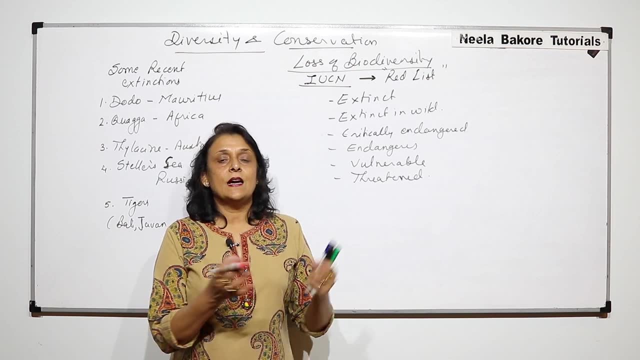 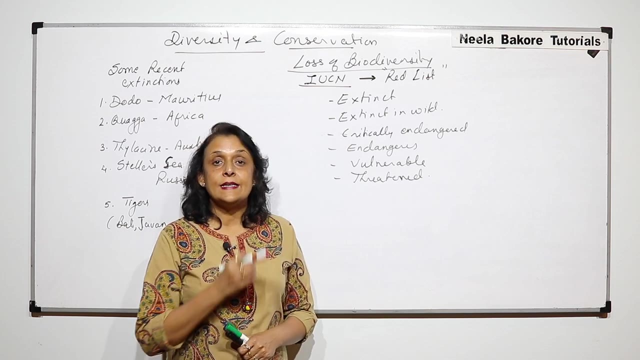 but there are few surviving in captivity, Like when we know that the animals are on the verge of getting extinct, we start conserving them And they may die in the nature, but maybe one or two still exist in captivity, maybe a zoo. 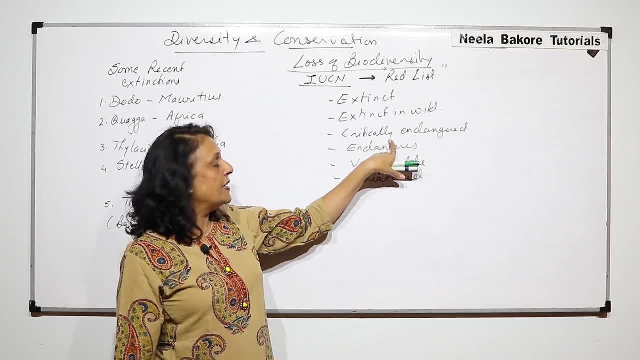 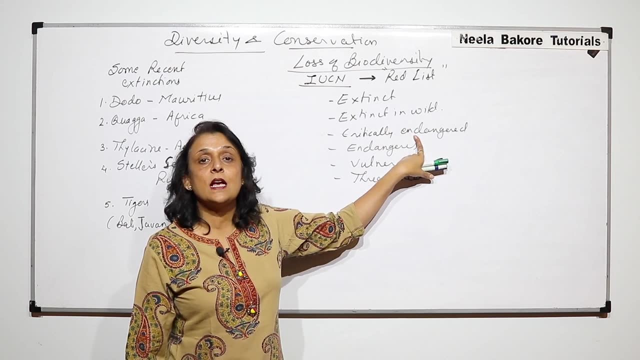 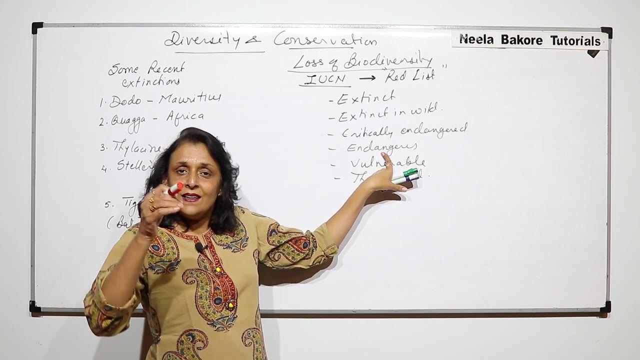 So then they are placed in this category. Critically endangered means: if you do not do anything or if strict measures are not taken, they will come in this category. So they are critically endangered animals. Then a little lower risk that they are endangered. 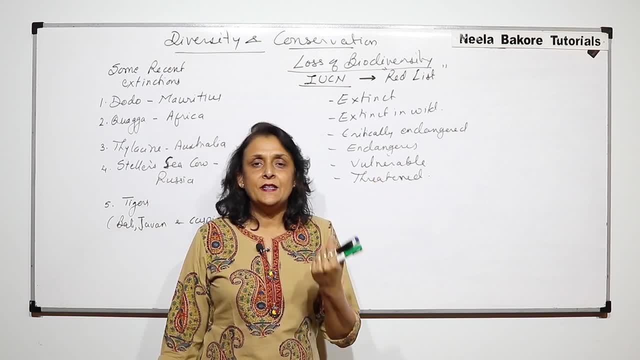 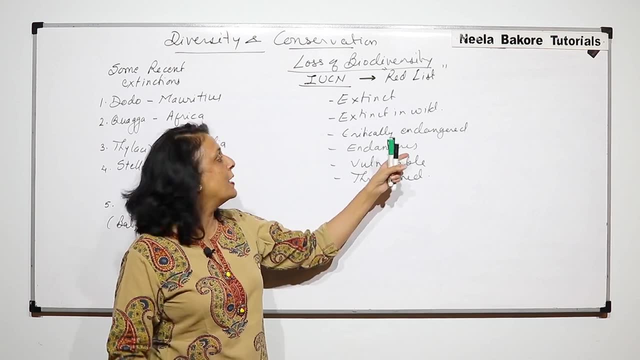 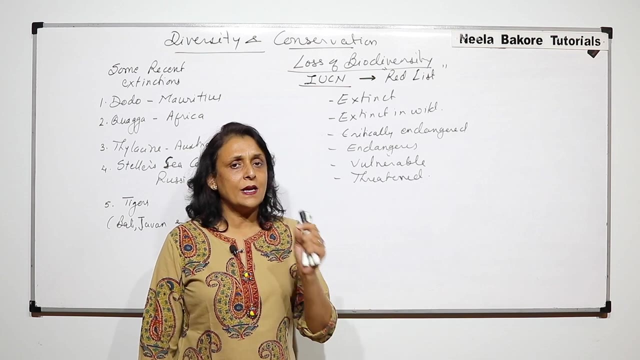 but you know we still have time. If we take simple measures also, we can protect these animals Vulnerable. they are at a risk of becoming endangered, Threatened. there are species which are killed for various reasons, So there is a threat for that. 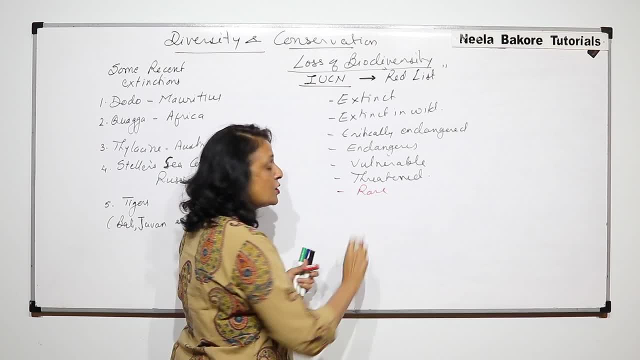 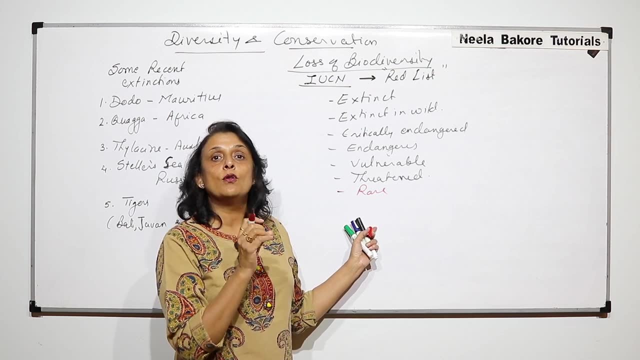 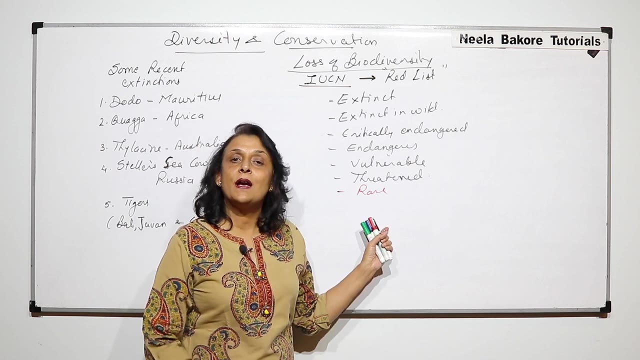 And then there is which is called a rare species. These rare means they are isolated in a particular area, No other area in the world, And if we do not take some measures to conserve them and if that area gets affected, then those species will become extinct. 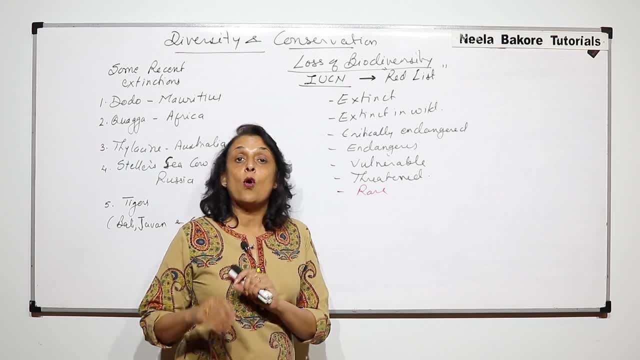 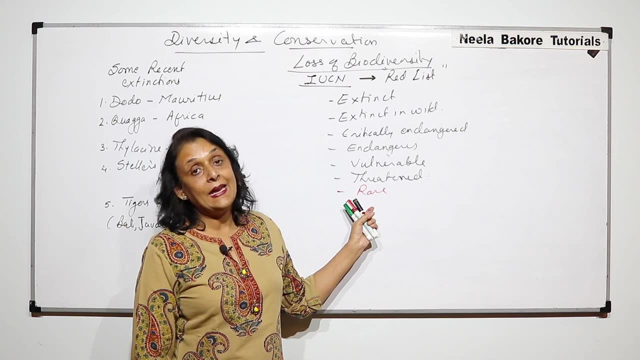 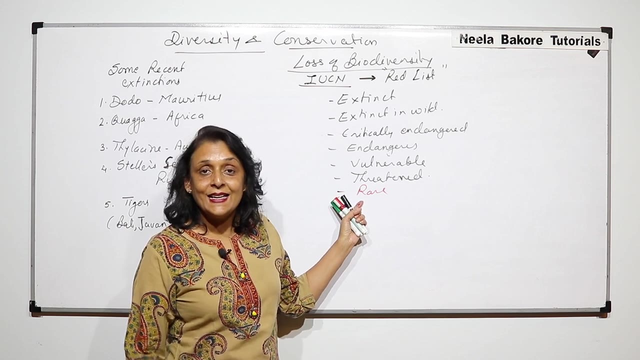 For example, if we talk about Australia kangaroos or marsupials, they are restricted only that area. They are in that zone. They are rare animals And if something goes wrong in that particular area and if marsupials become extinct from that area, 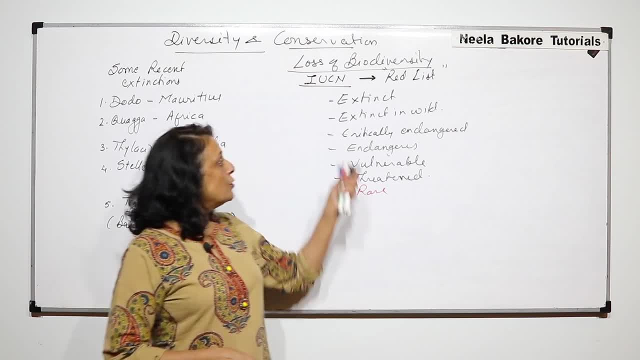 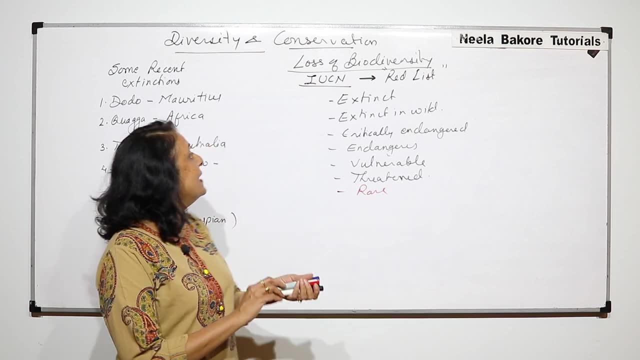 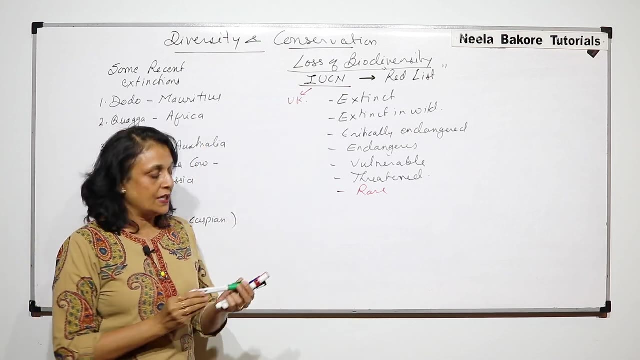 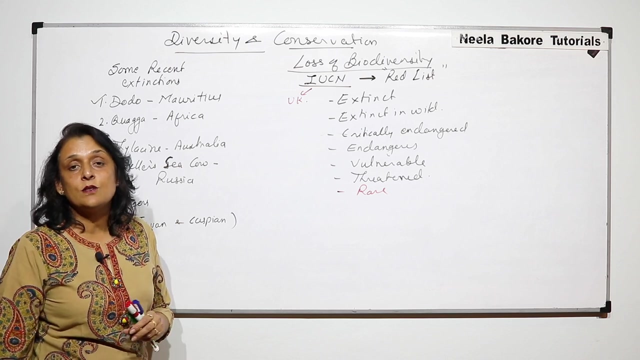 that means they will be gone from this world. So these are various categories in which the animals are classified. The list is updated, The headquarter is in UK And, according to the recent extinctions, we have few names here. Dodo, which was a flightless bird. 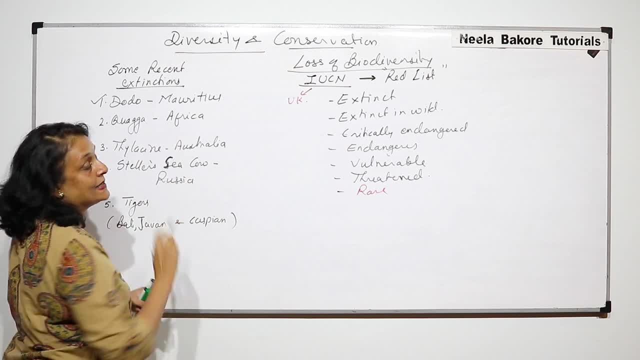 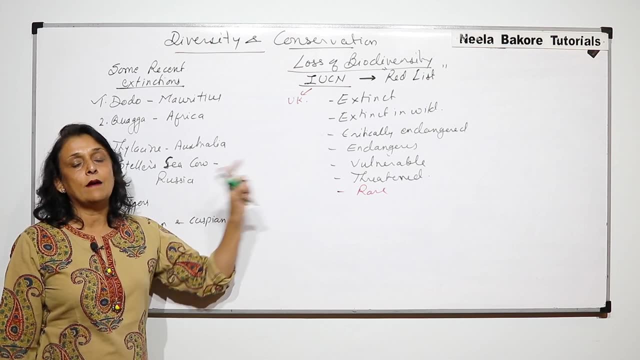 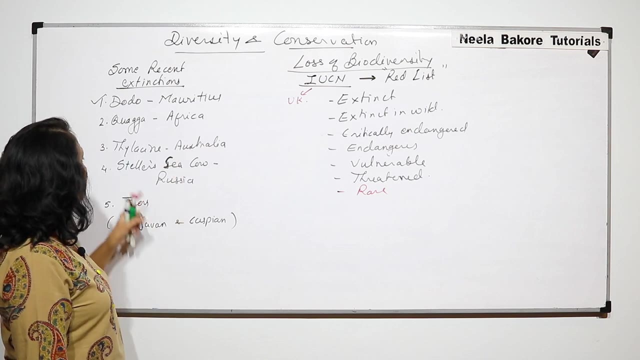 And I am using was because now they are all extinct. So dodo was a flightless bird which was found in Mauritius. We will take this example again after we come to the causes. Quagga was a zebra-like animal found in Africa. 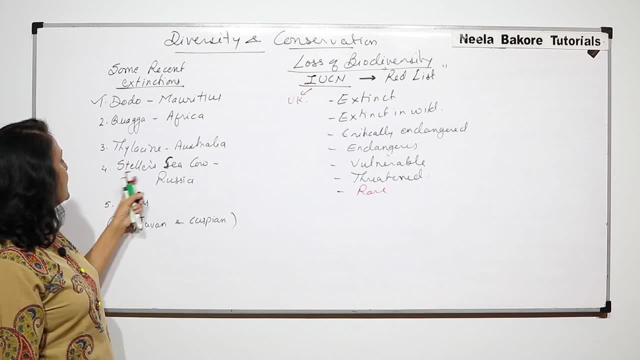 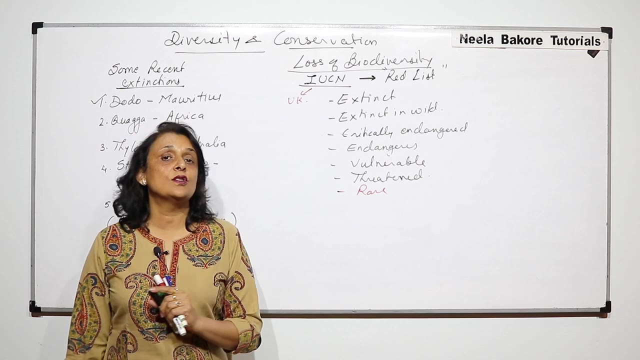 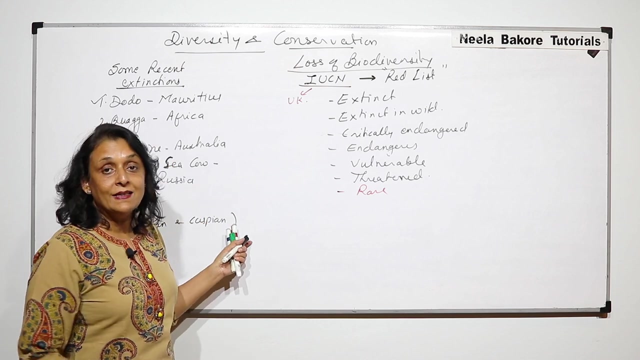 Thylacine in Australia, Stellar sea cow, Russian And three different types of tigers: Bali, Javan and Caspian. These are the recent extinctions which have taken place, And when we say recent, it is like in last 40-50 years. that is recent. 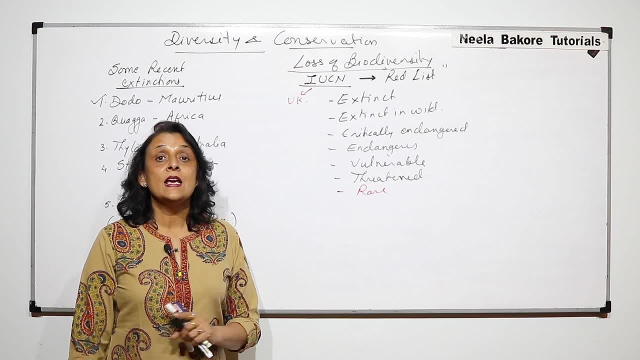 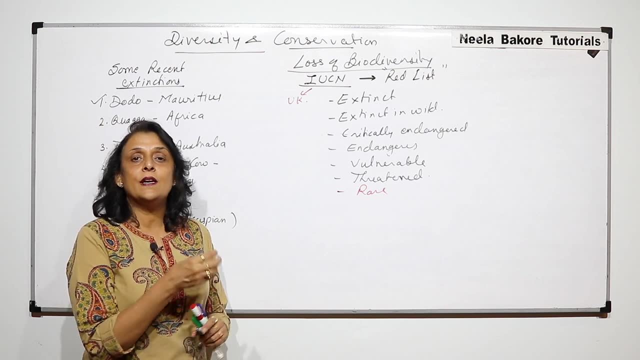 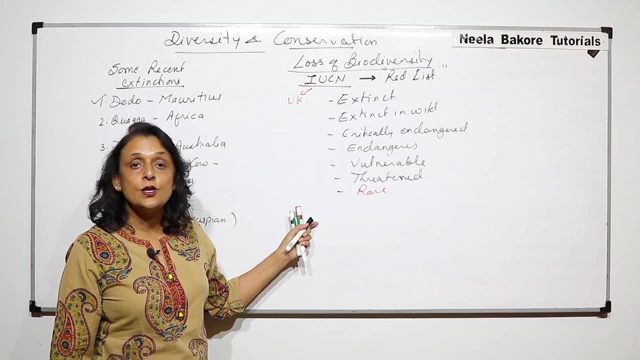 Because when we talk of living organism and biodiversity, our time period is of thousands of years or maybe millions of years. So in that millions of year time period, 30-40 years is like a very short period of time. So these are the categories in which the red list includes various animals. 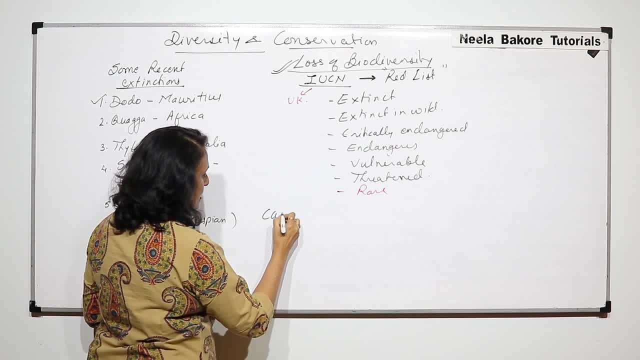 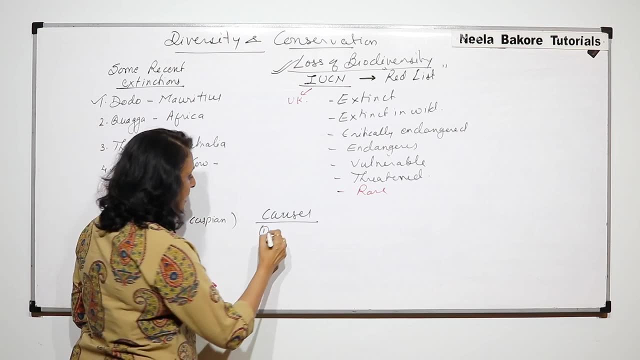 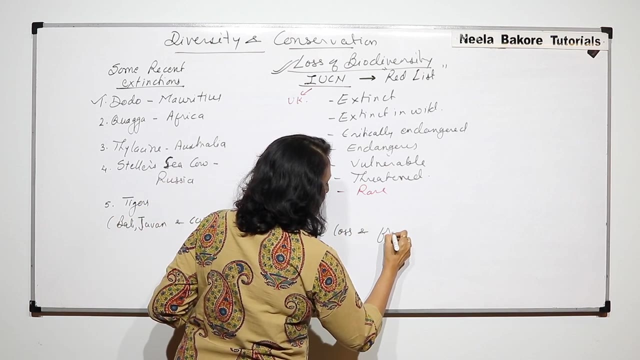 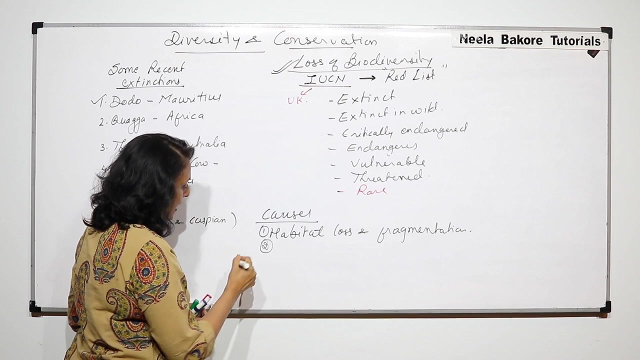 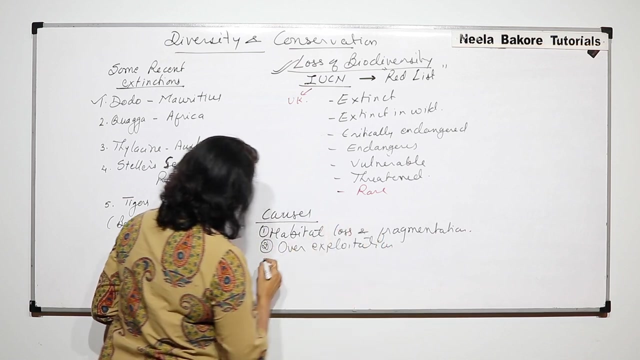 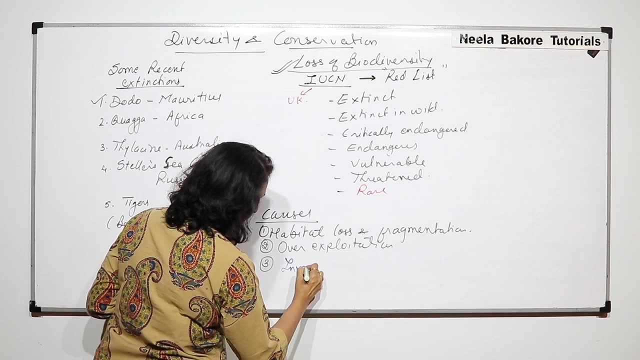 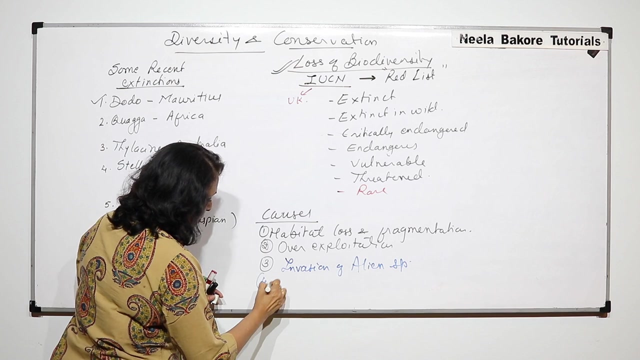 Now, what are the reasons, the causes of this loss of biodiversity? The first is habitat loss And fragmentation. The second cause is over exploitation. Third is invasion of alien species And the third cause is over exploitation. And the fourth is co-extinction. 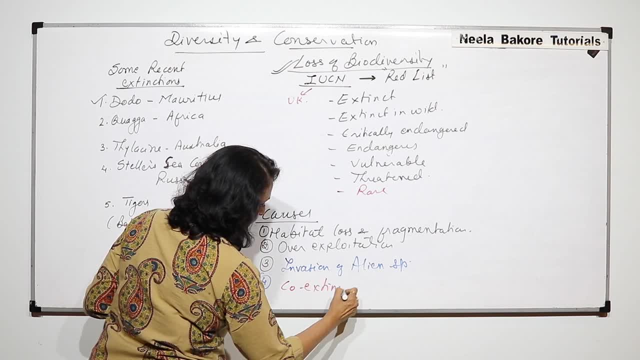 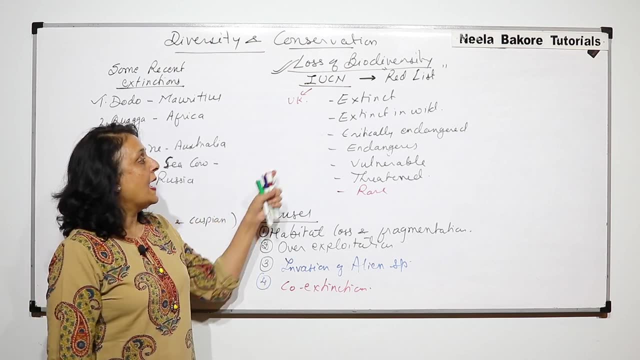 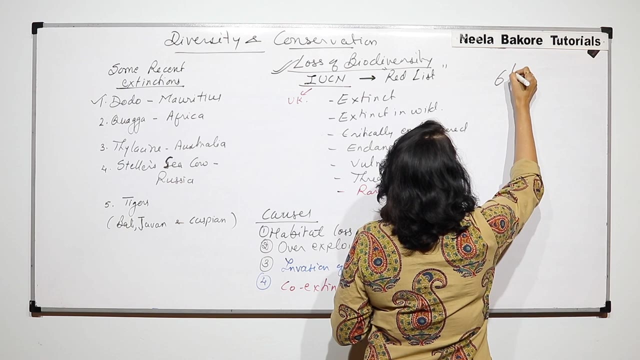 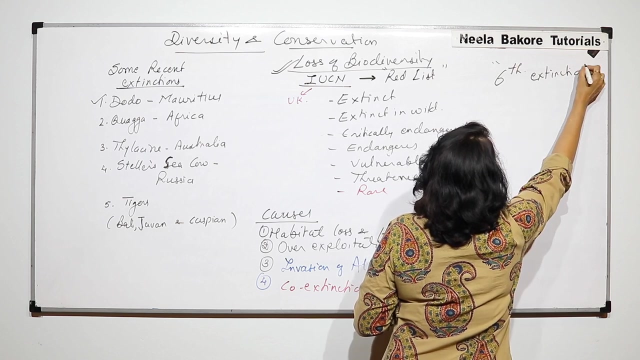 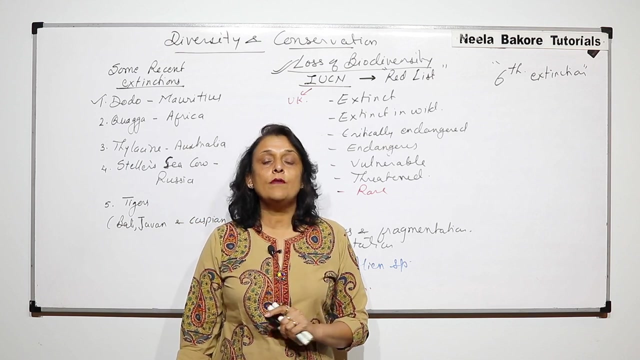 These are the four main causes of extinction, And the extinction which is taking place nowadays, or in this particular time, is the sixth major extinction. That means five such extinctions have taken place already. One which we are aware of is when dinosaurs they got extinct. 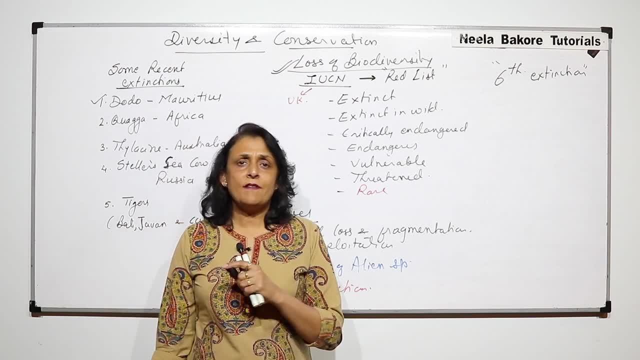 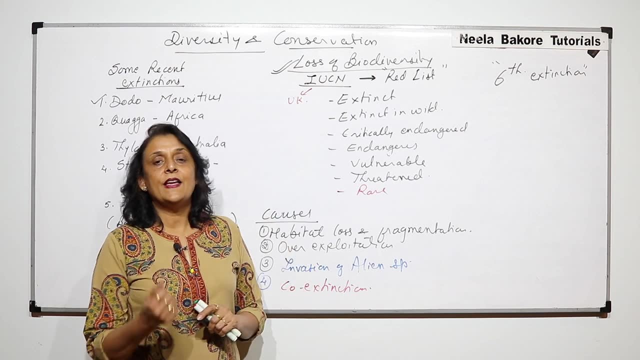 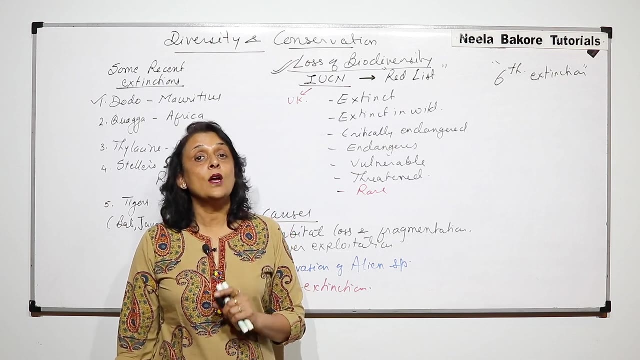 This was like a major thing. Now there are various theories on the reasons why dinosaurs got extinct. Some scientists believe that it was the climatic change. Dinosaurs were reptiles And reptiles are cold blooded animals, So probably they were not able to cope up with the temperature change. 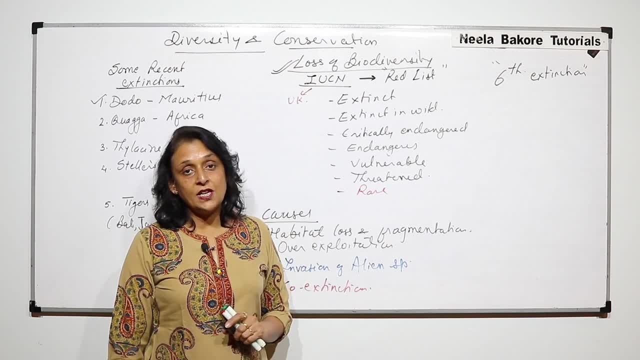 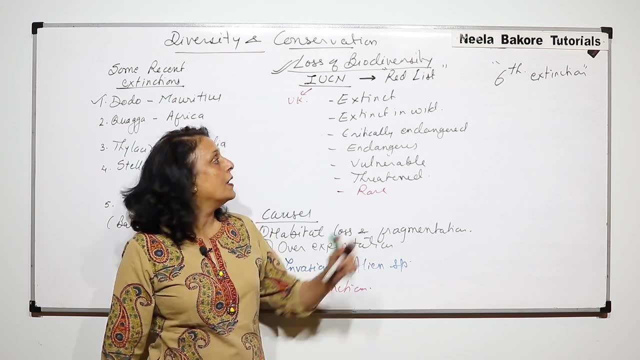 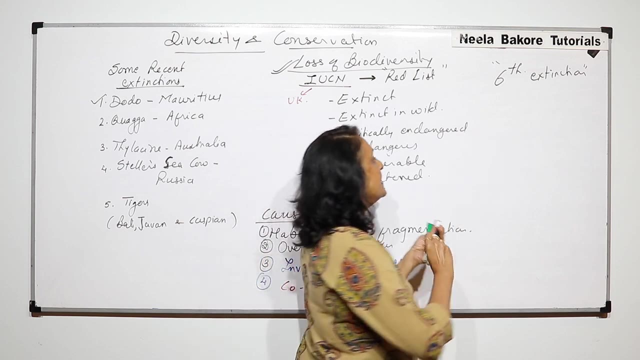 Some believe that there was change in the vegetation and they could not find the food which was required for them. So, whatever the reason was, it was natural. But the sixth extinction which is taking place right now is having a different reason, And this is due to human activities. 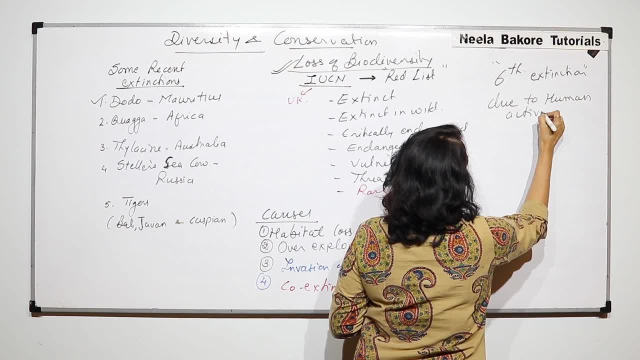 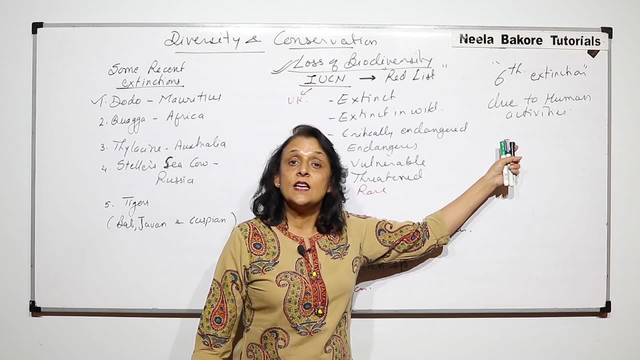 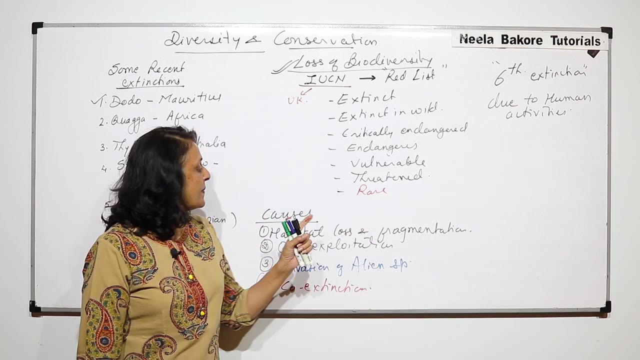 So we call it anthropogenic activities. So the reason for the sixth one is totally different. The five earlier ones were due to some or the other natural reasons, And we have to talk about these four main causes of extinction. Let us talk about the first. 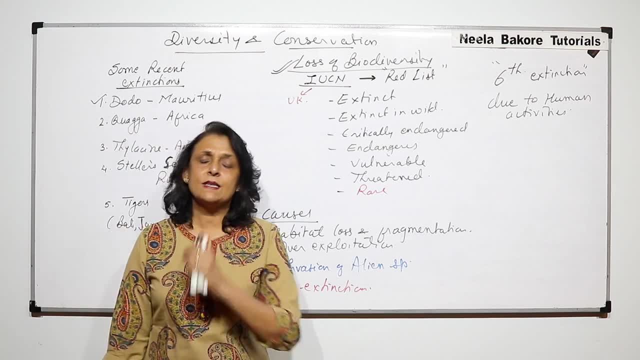 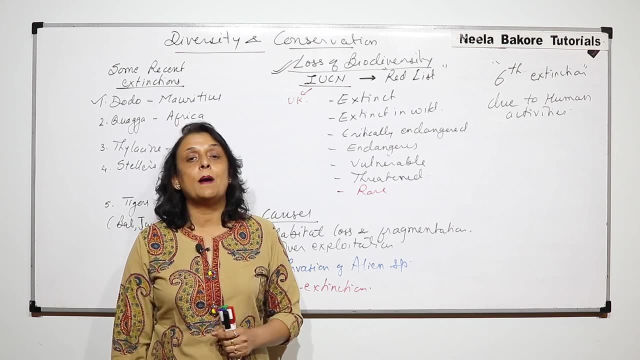 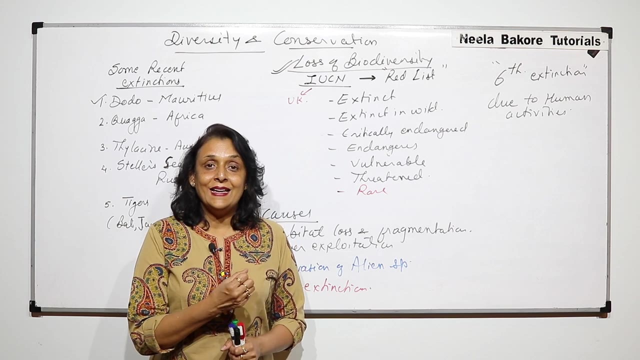 What exactly we mean by habitat loss. We will take a simple example. Nowadays in the newspaper there are articles which are talking about that. the wild animals are entering into villages. Wild animals are killing the domestic animals. They are entering into the houses and carrying the small babies who are sleeping there. 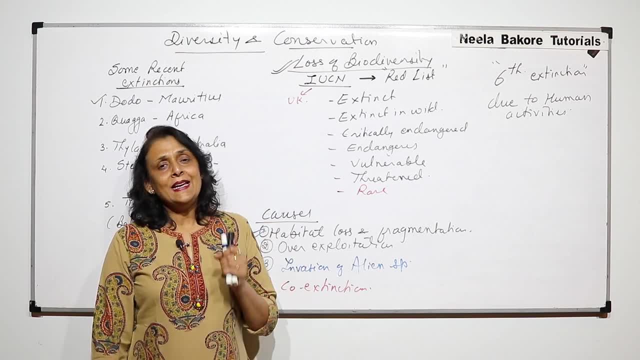 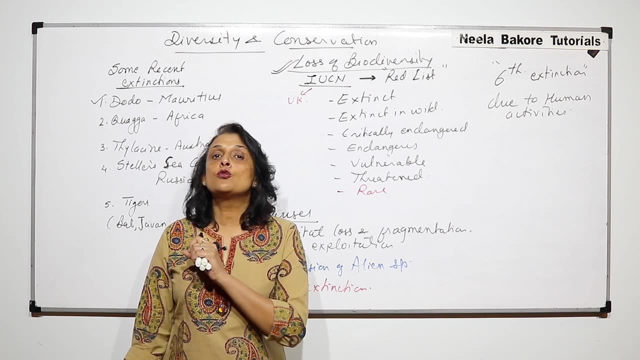 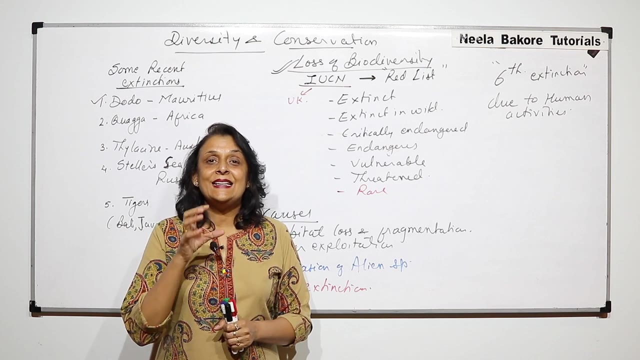 Or attacking people in the village And they say that the tigers or lions, they are entering into human habitation. The statement is totally wrong. Where is this habitation? Where is this village? The village is in the territory of these animals. 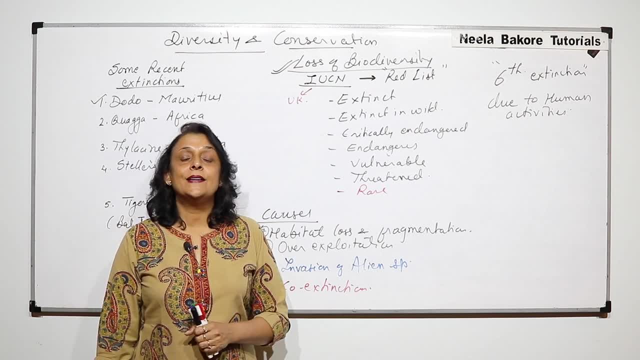 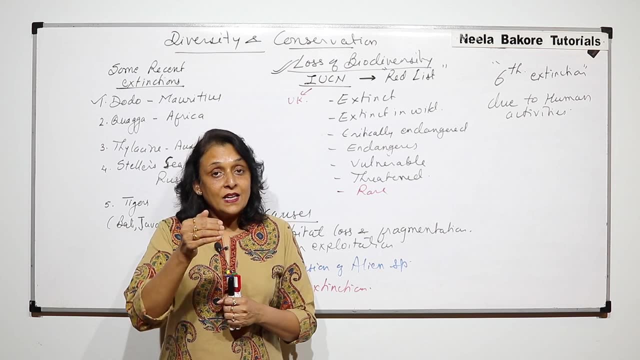 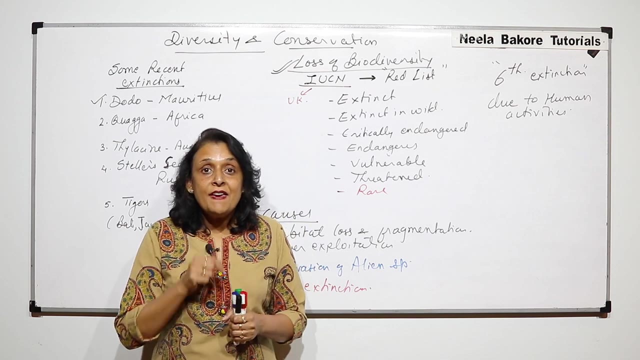 These big cats, like lions and tigers, their territories are like in kilometers And because we are living there, we are giving this land to the villagers for farming and making their huts there. We have invaded in their territories. So and if we want to live there, 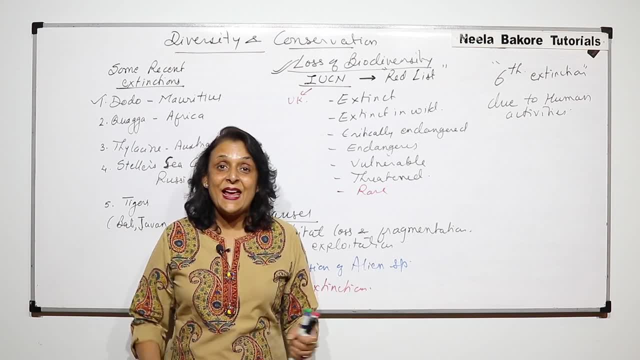 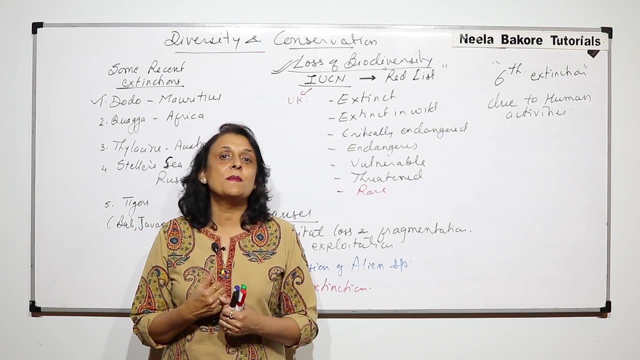 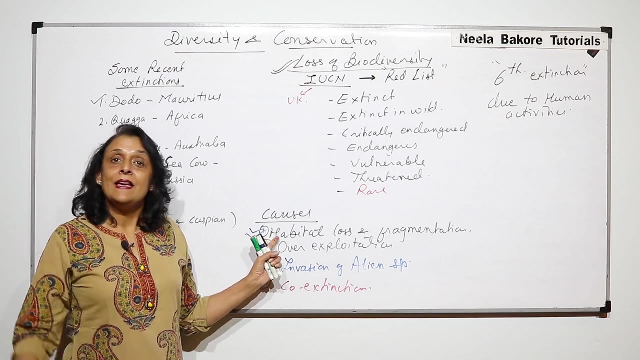 we are going to cut forests, we are going to make that land plain for us so that we can grow crops there. So we have entered into their territories. They are not coming out of their territory and coming into our villages. So it is loss of their habitat and they are roaming into their territory only. 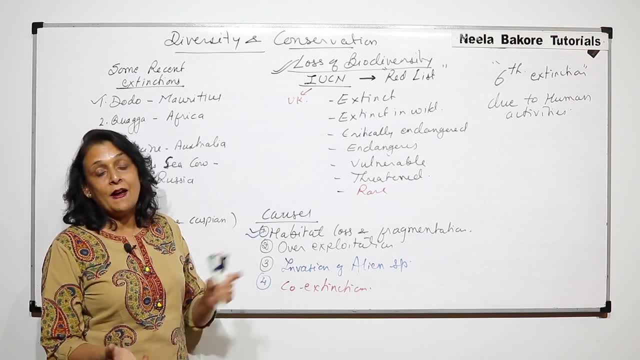 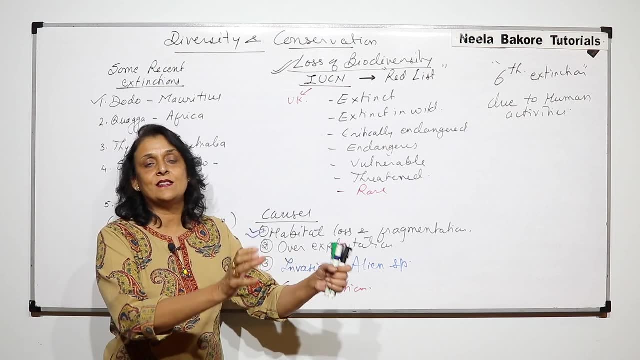 The village comes into their territory and if they find an easy kill, if a domestic animal is there who is tied with a rope and is like in a particular area, then it is an easy kill for these animals. And if they get easy kills, 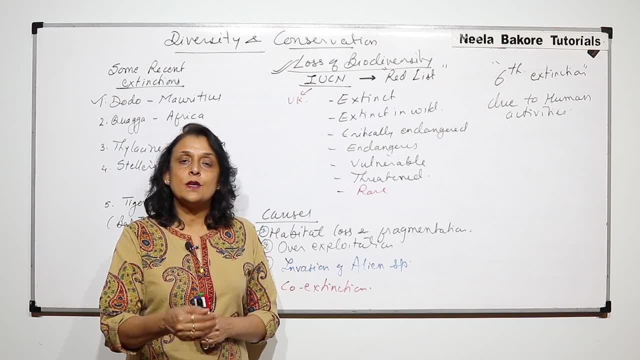 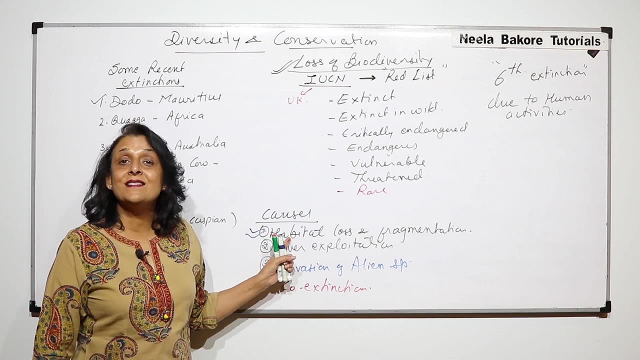 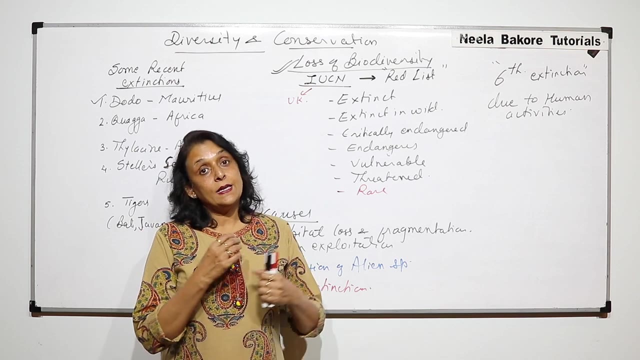 why would they work harder So every time? they will keep visiting that village and kill some animal or maybe a human. So it is their habitat loss. Fragmentation is we have broken their habitat into parts. There was a news recently that a big national park 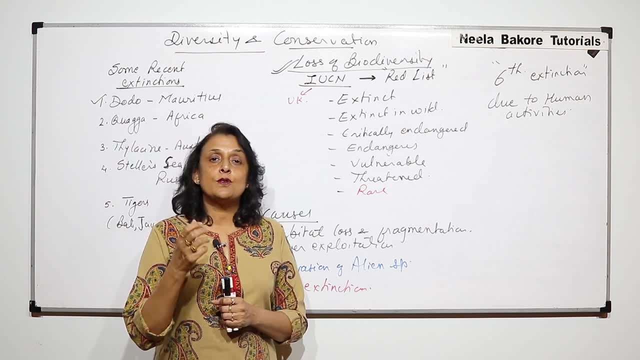 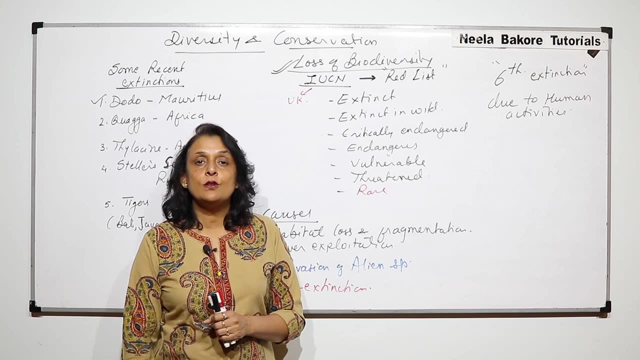 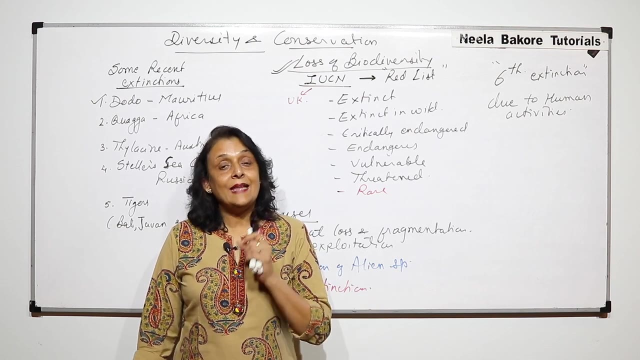 because of this industrialization and because of this human habitation, they had to construct a road, and this road was passing through that national park. So, basically, you have divided their habitat into two pieces. This is fragmentation, and these animals, they run away from humans.